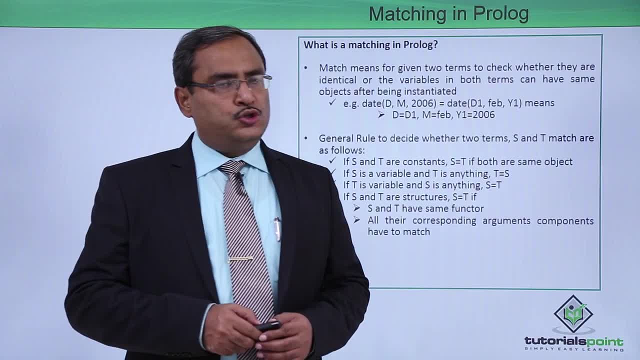 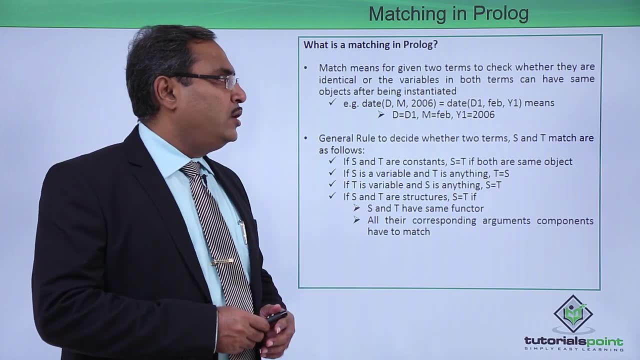 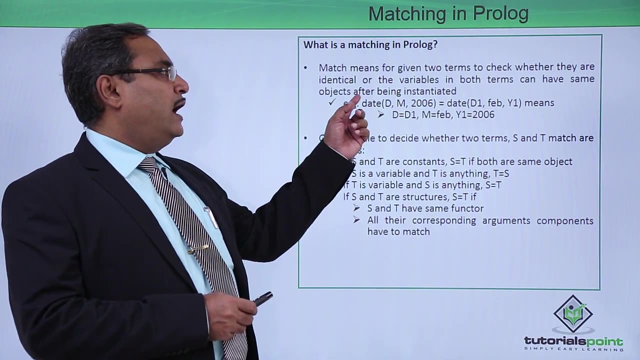 Let us discuss matching in prologue. So here is the respective text for our discussion. Match means for given two terms to check whether they are identical or the variables in both terms can have the same objects after being instantiated. Let us go for example that will: 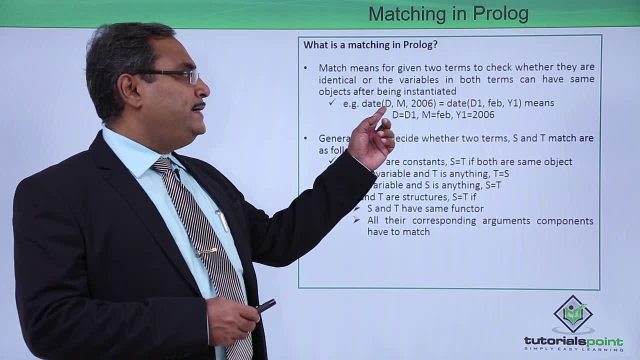 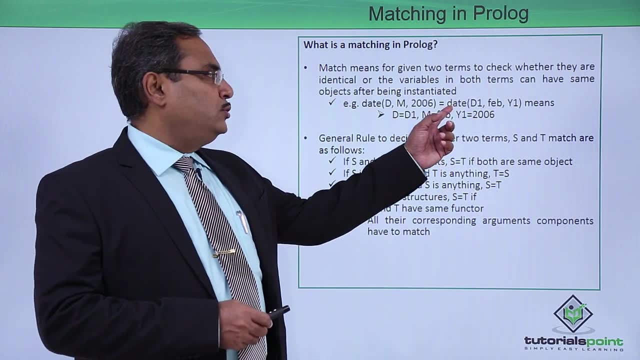 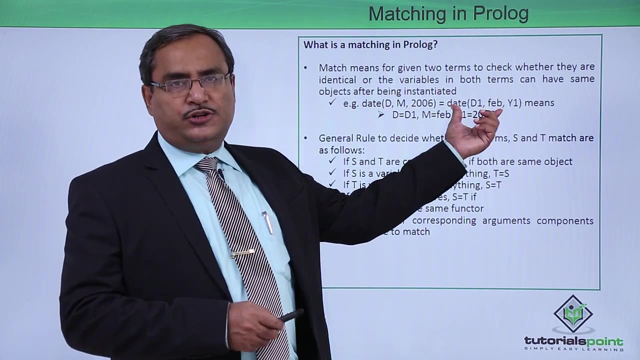 clear our doubts. As example, det, dm- they are the variables because they are written in capital letters. 2006 is equal to det d1. fav y1 means. So if we write this, equal to, in between this structure, this another structure, both are of type dets and here it is defined. 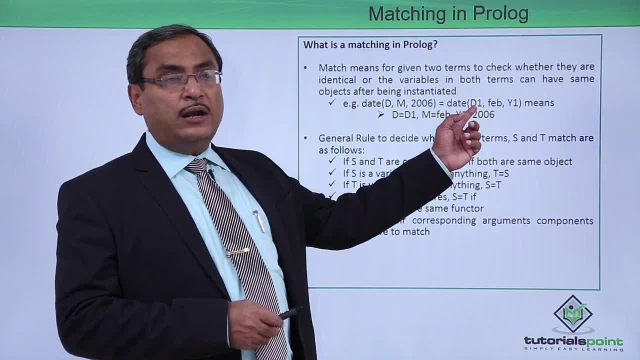 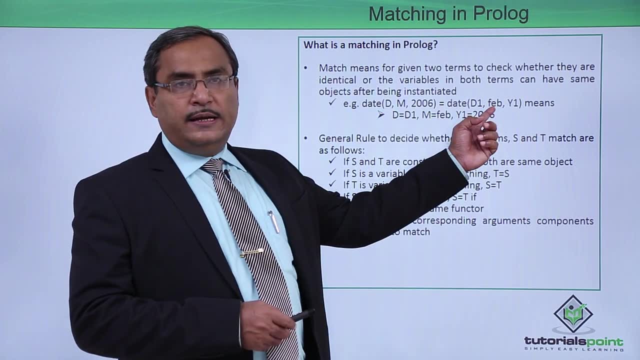 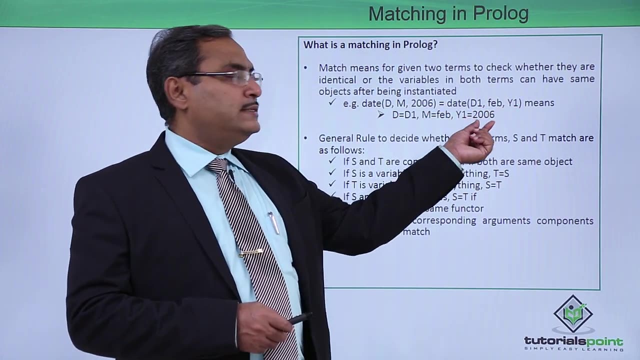 as here is written as d and here it is written as d1.. So it means that d is equal to d1, fav. Here it is written as variable m and here it is written as fav, So m is equal to fav. Here it is 2006,. here it is y1.. So y1 is equal to 2006.. General rule to decide. 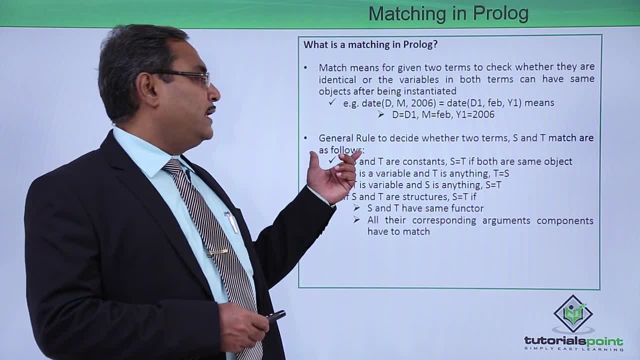 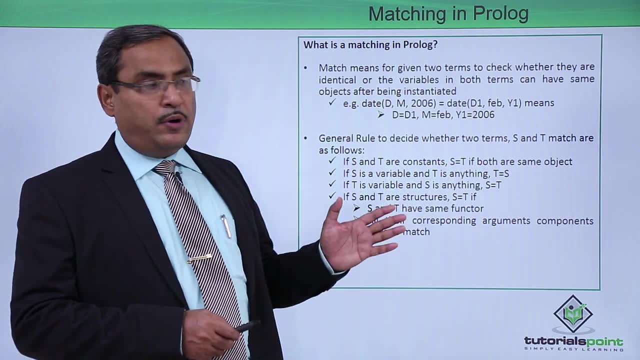 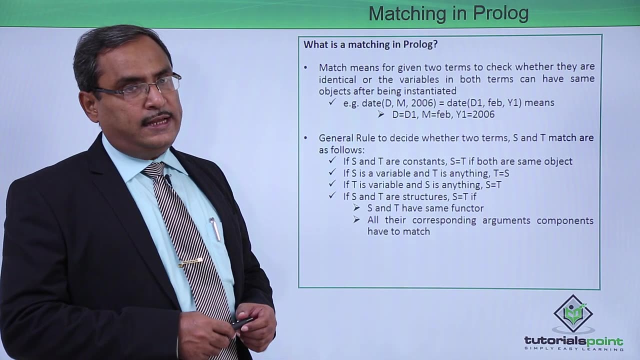 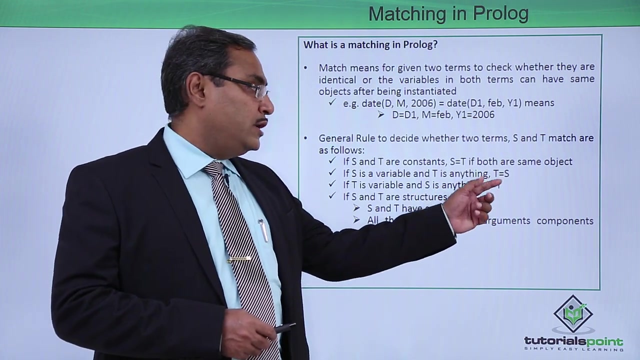 whether two terms, s and t, match, are as follows: If s and t are constants, s is equal to t. if both are same object, If s is a variable and t is anything, then t is equal to s. in that case, If t is a variable and s is anything, then s is equal to t. So 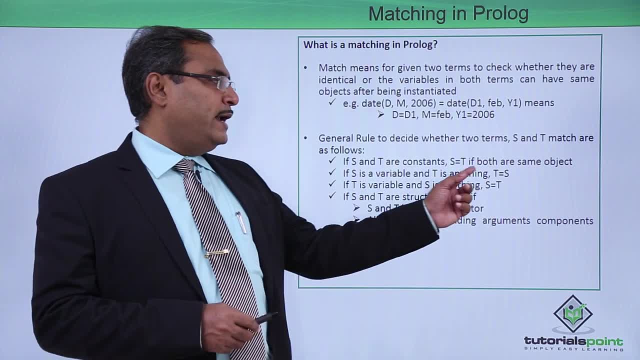 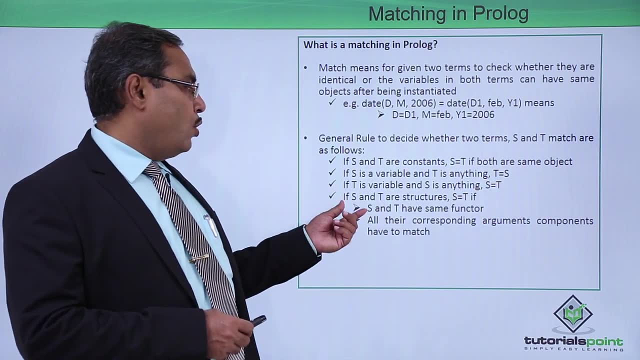 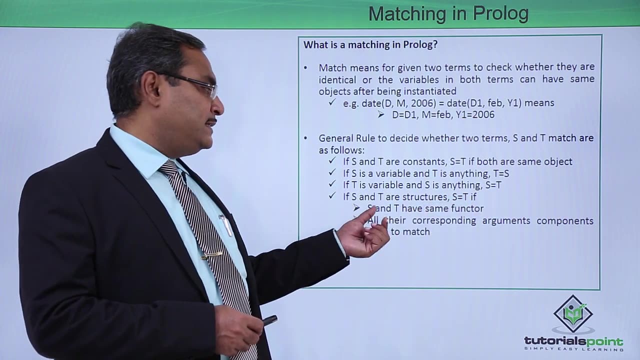 that is just opposite one. So here s is a variable, So we are writing this one. t is equal to s. Here t is a variable, So we are writing this one, as s is equal to t If s and t are structures and s is equal to t if s and t have same functor, functor and function. 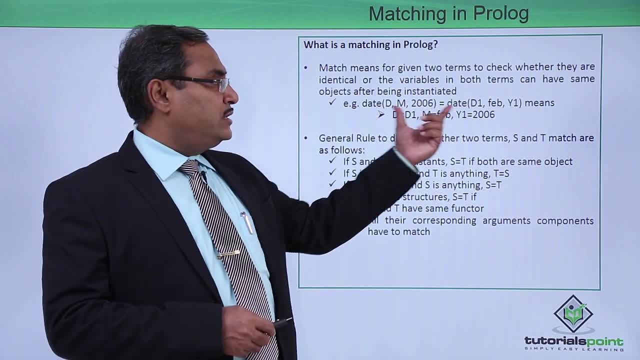 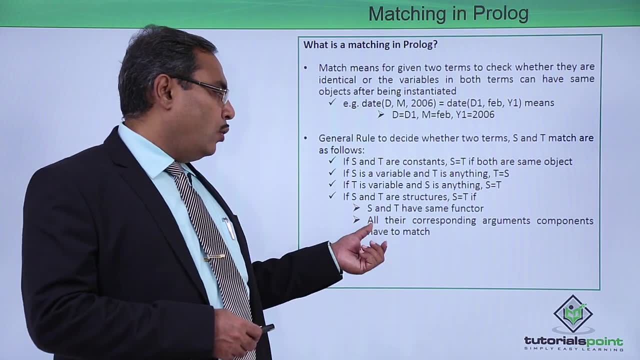 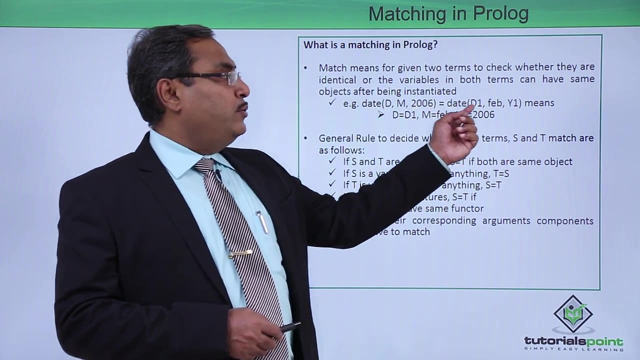 means this date will remain the same, Because this is a structure. this is a structure, so when you are writing equal to, then this functor must be same. All their corresponding arguments, components, have to match. So here we are having three components. here we are having 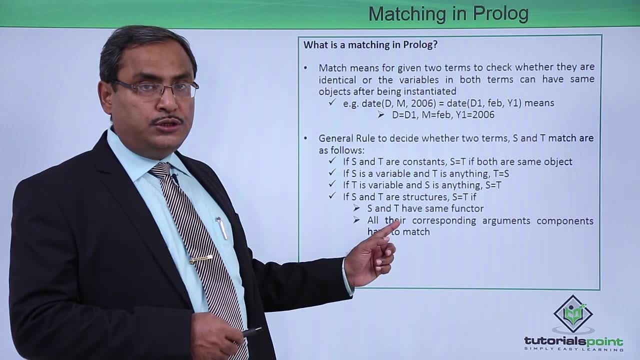 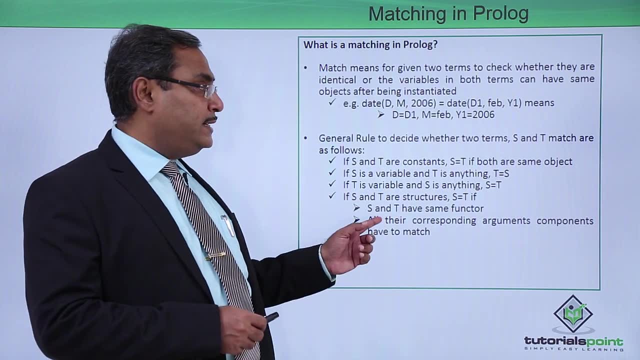 three components, So one by one, they should match. So in this way we have discussed what is a matching in prologue. I think you are getting this idea with these examples And all such discussions. Thanks for watching this video.